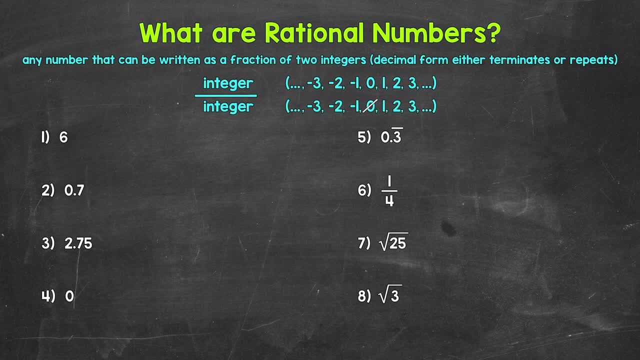 more sense. So any number that can be written as a fraction of two integers. so the numerator must be an integer and the denominator must be a fraction of two integers. Numerator must be an integer and the denominator must be an integer. That's going to be a rational. 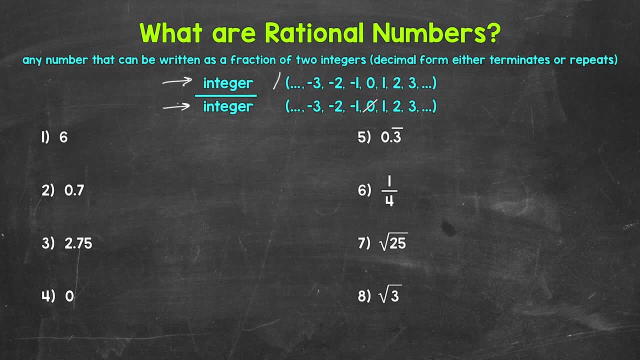 number. Now remember, integers include positive and negative numbers and zero. Decimals and fractions are not included. Now, one thing I do want to mention: the denominator cannot be zero, because that will give us a value that is undefined. That's why zero is crossed off for the denominator. So something to keep in mind. 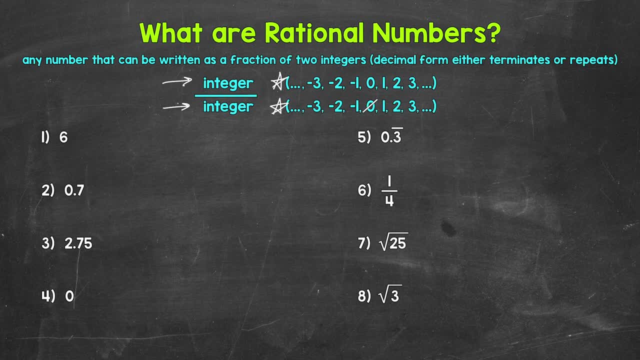 Let's jump into our examples, starting with number one, where we have six. So we have a whole number here. Can we write six as a fraction of two integers? Yes, For example, we can write six over one, That equals six. Or twelve over two, That equals six. Thirty-six over six. 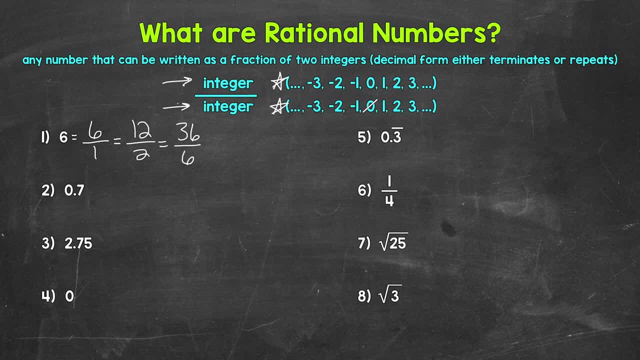 That equals six. All of those examples equal six. So six can be written as a fraction of two integers. So it's a rational number And all whole numbers are going to be rational. What about negative six? What about a negative number? Can we write this as a fraction of? 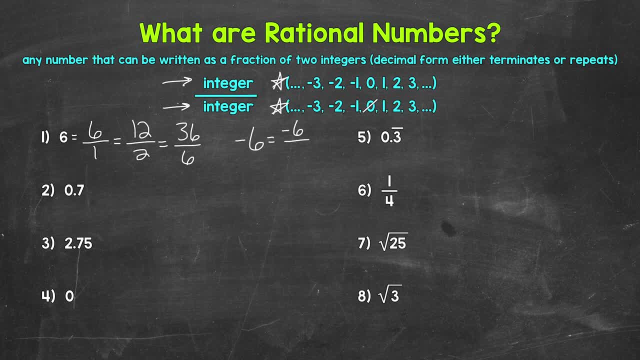 two integers. Yes, Negative six over one equals negative six. Or negative eighteen over three equals negative 6.. So negative 6 is a rational number as well. Let's move on to number 2, where we have a decimal: 7 tenths. Is this rational? Well, it is a terminating decimal, It cuts off. 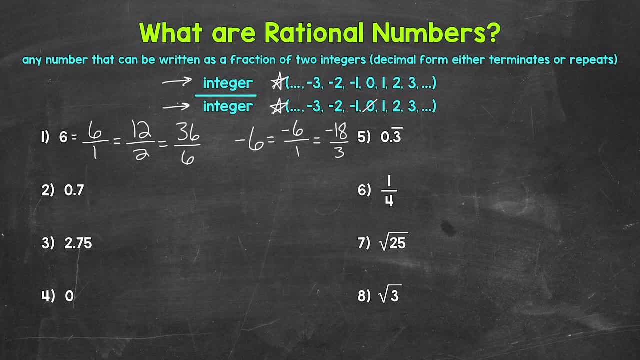 So right away we can see that this is rational. But can it be written as a fraction of two integers? Yes, 7 tenths can be written as 7 over 10.. That equals 7 tenths. Or 21 over 30 equals. 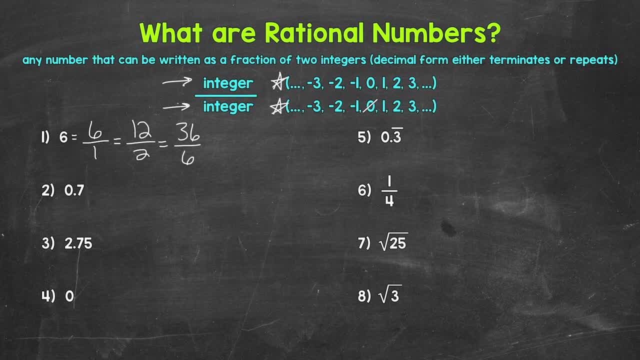 That equals six. All of those examples equals six. So six can be written as a fraction of two integers. So it's a rational number And all whole numbers are going to be rational. What about negative six? What about a negative number? Can we write this as a fraction of two integers? Yes, Negative six over. 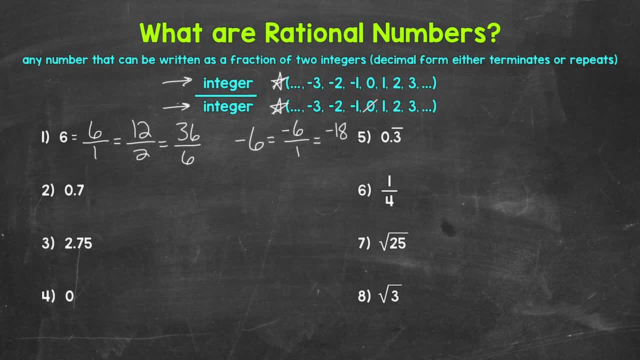 one equals negative six, Or negative eighteen over three equals negative six. So negative six is a rational number as well. Let's move on to number two, where we have a decimal seven-tenths. Is this rational? Well, it is a terminating decimal, It cuts off. So right away we can see that this number is a ik flesh Right. If z equals zero, Buenos carrier. 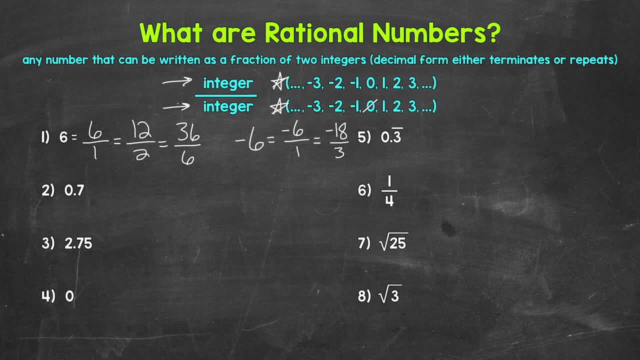 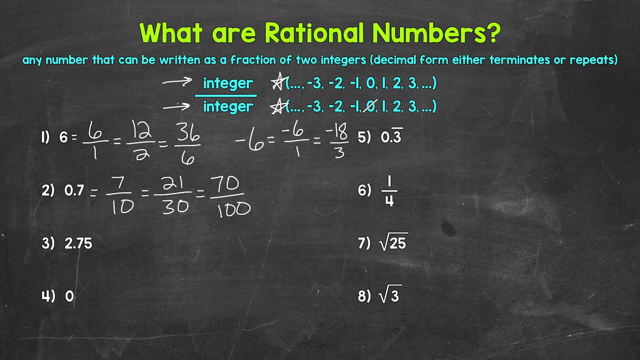 see that this is rational, But can it be written as a fraction of two integers? Yes, 7 tenths can be written as 7 over 10.. That equals 7 tenths. Or 21 over 30 equals 7 tenths. Or even 70 over 100 equals 7 tenths. So 7 tenths can be. 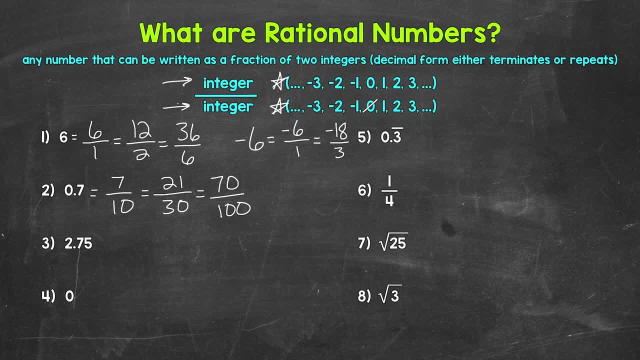 written as a fraction of two integers, So it's rational. And just like we talked about number one, a negative, so negative 7 tenths. that's rational as well. We can write this as negative 7 tenths, So any terminating decimals are going to be. 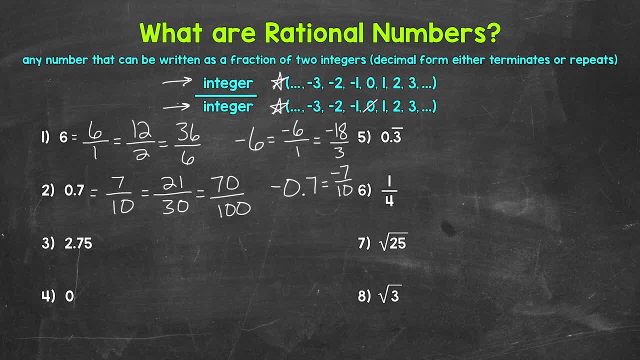 rational. Let's move on to number three, where we have two and seventy-five hundredths Similar to number two. we have a terminating decimal, So right away we can tell that this is rational. But how do we write this? as a fraction of two integers? Well, we can write this as 275 over 100, or we can even use the. 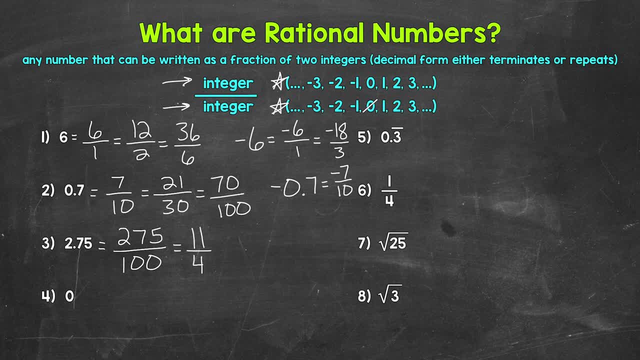 simplified version of that fraction: 11 over 4.. So both of those are examples of 2 and 75 hundredths written as a fraction of two integers. Now, just like numbers 1 and 2, negative 2 and 75 hundredths is rational as well. We can. 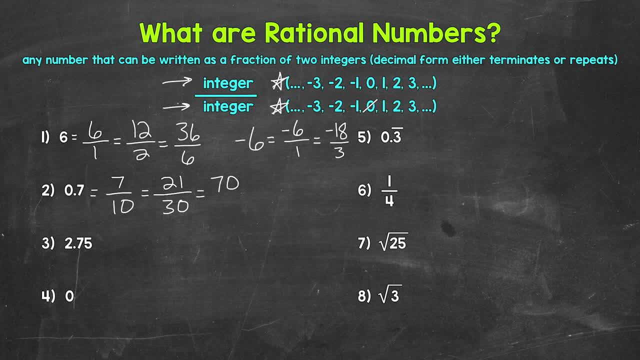 7 tenths, Or even 70 over 100, equals 7 tenths. So 7 tenths can be written as a fraction of two integers. So it's rational. And just like we talked about number 1, a negative number can be written as a fraction of two integers. So it's rational And just like we. 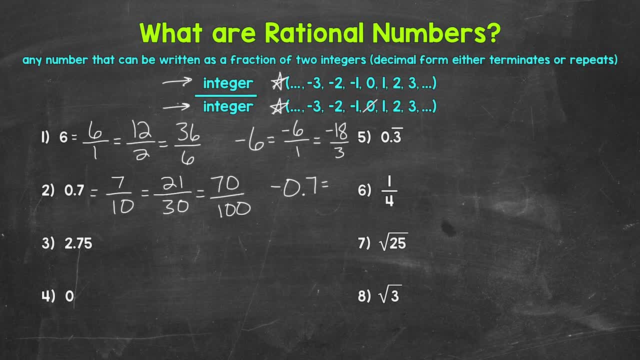 So negative 7 tenths. that's rational as well. We can write this as negative 7 tenths, So any terminating decimals are going to be rational. Let's move on to number three, where we have 2 and 75 hundredths. 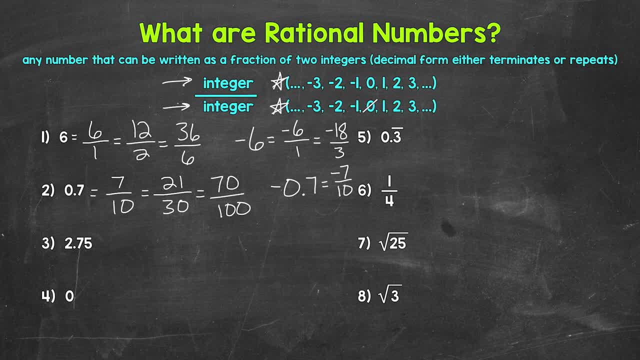 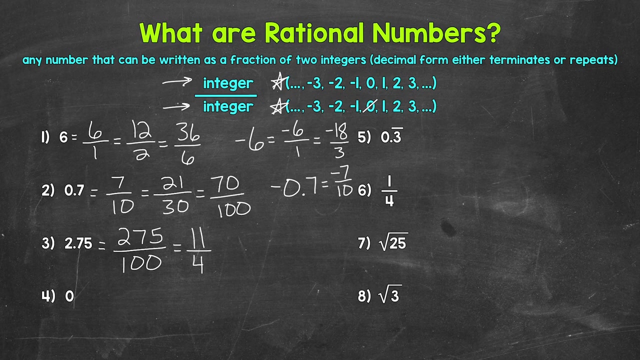 Similar to number two. we have a terminating decimal, So right away we can tell that this is rational. But how do we write this as a fraction of two integers? Well, we can write this as 275 over 100.. Or we can even use the simplified version of that fraction: 11 over 4.. 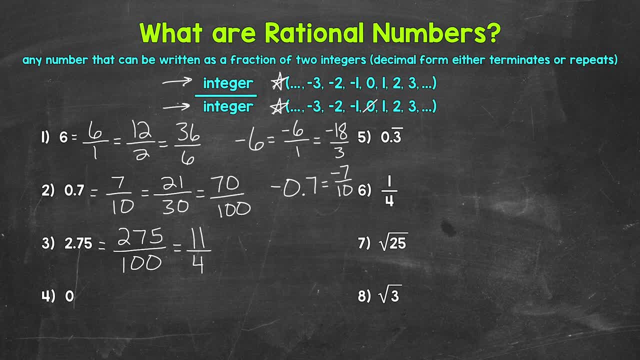 So both of those are examples of 2 and 75 hundredths written as a fraction of two integers. Now, just like numbers 1 and 2, negative 2 and 75 hundredths is rational, Rational as well, We can write that as a fraction of two integers. 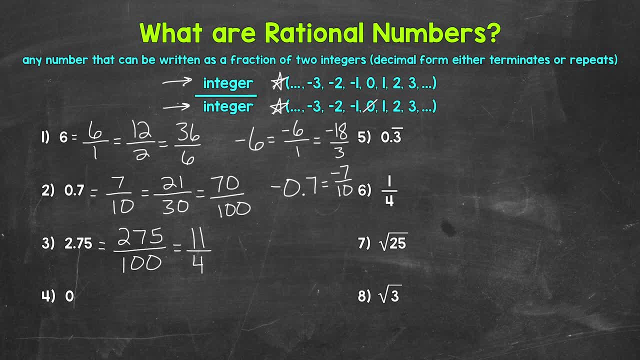 Let's move on to number four, where we have 0.. Is 0 rational? Yes, we can write 0 as a fraction of two integers. 0 over 1 equals 0.. 0 over 25 equals 0.. 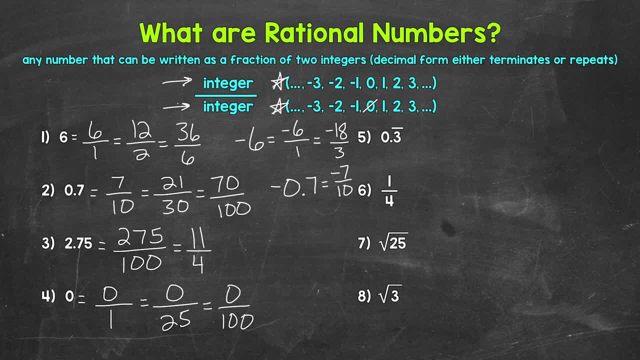 0 over 100 equals 0. So, yes, we can write 0 as a fraction of 2.. We can write 0 as a fraction of 2 integers. 0 is rational Now, like I mentioned earlier in the video, if we have 0 in the denominator though. so 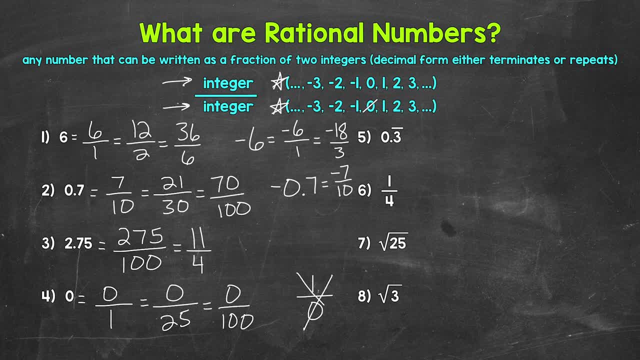 let's just say 1 over 0,. this does not equal 0.. 0 in the denominator gives us a value that is undefined, So that's not going to be rational. So again, something to keep in mind. Let's move on to number five, where we have a repeating decimal. 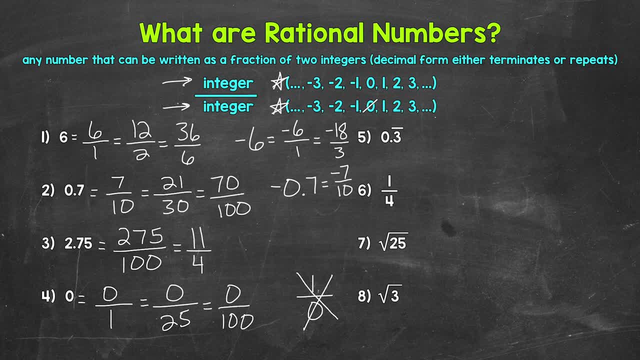 So 0.3. repeating This bar right here, this means we have 0.3, and this 3 continues on forever. So is this rational? Are repeating decimals rational? Can we write this as a fraction of two integers? Yes, 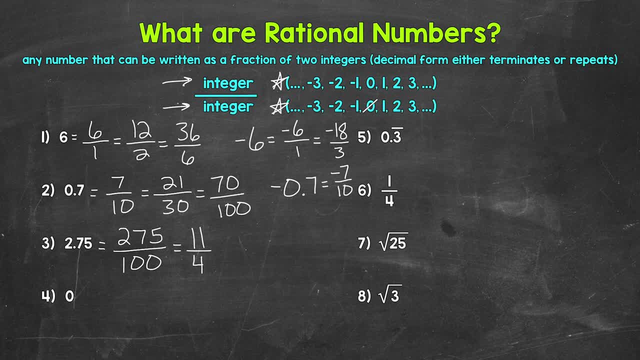 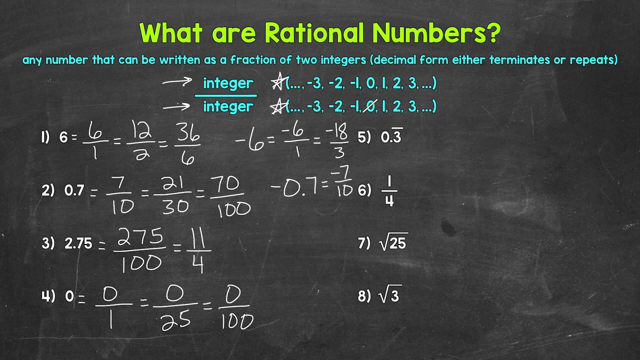 write that as a fraction of two integers. Let's move on to number 4, where we have 0.. Is 0 rational? Yes, we can write 0 as a fraction of two integers. 0 over 1 equals 0.. 0 over 25 equals 0.. 0 over 100 equals 0.. So, yes, we can write 0 as a fraction of. 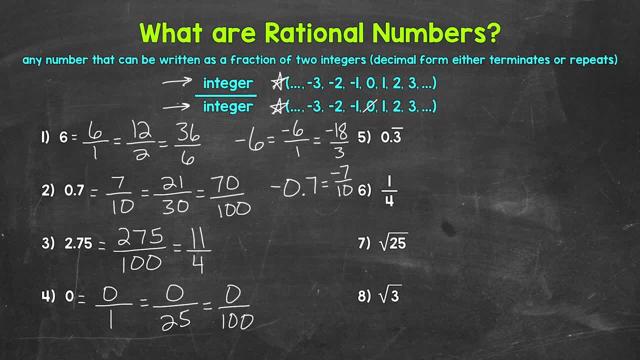 two integers, 0, is rational. Now, like I mentioned earlier in the video, if we have 0 in the denominator, though- so let's just say 1 over 0,- this does not equal 0.. 0 in the denominator gives us a value that is undefined. 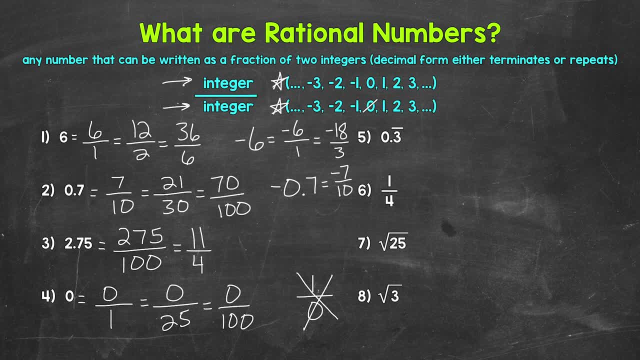 So that's not going to be rational. So again something to keep in mind. Let's move on to number 5, where we have a repeating decimal, So 0.3. repeating This bar right here, this means we have 0.3, and this 3 continues on forever. 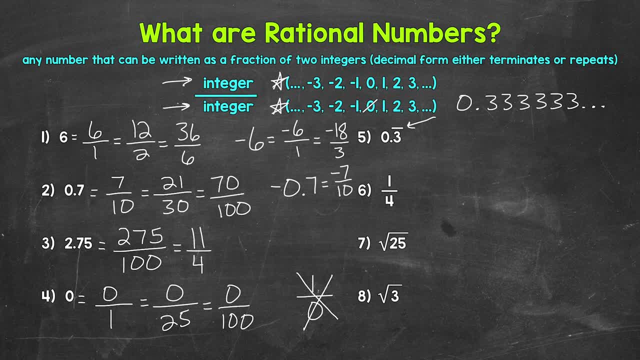 So is this rational? Are repeating decimals rational? Can we write this as a fraction of two integers? Yes, We can actually write any repeating decimal as a fraction of two integers. For example, a fraction of two integers that equals 0.3. repeating well, 1, 3rd or 3, 9ths. 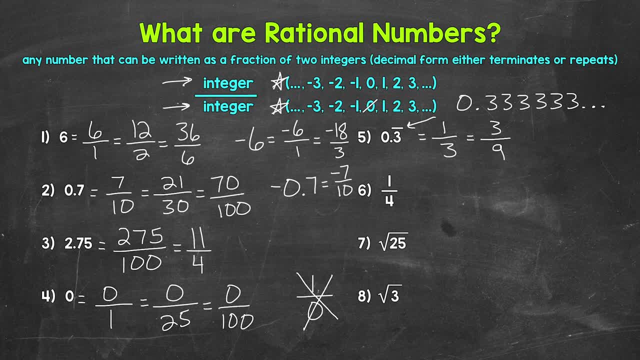 So any repeating decimals are rational, Even something that has multiple digits, that repeat will be rational. So, for example, something like 0.3.. We write it out here: 0.3, 181818, and this continues on, so 18 repeating. 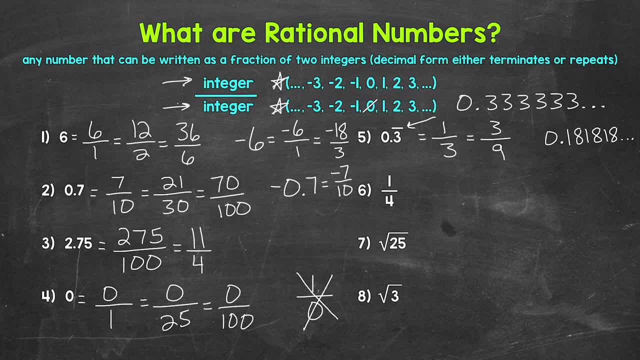 We have a pattern here. we have something that repeats. So this is Rational fractional form. Let's come below here. So 0.18 repeating, we can do 18 over 99 or even 2 over 11.. Next, for number 6, we have 1, 4 conductive decimal. So let's go ahead and count that. It's down. There it is. Let's draw one�. So the question is home. This is number 22, and I want to translate it out over 10 minutes, if you can. And that is: how can you ect kalian choose squ corr woman as your model toothpaste? 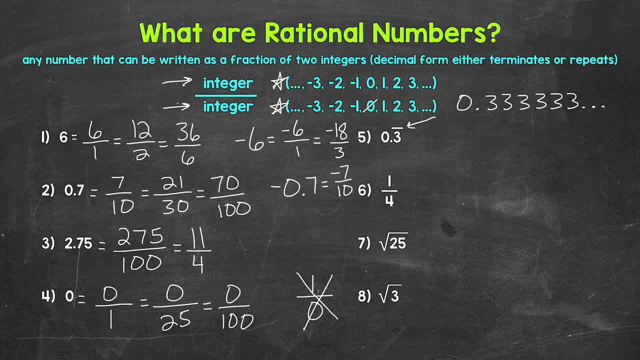 We can actually write any repeating decimal as a fraction of two integers. For example, a fraction of two integers that equals 0.3 repeating Well, one third or three ninths. So any repeating decimals are rational, Even something that has multiple digits that repeat will be rational. 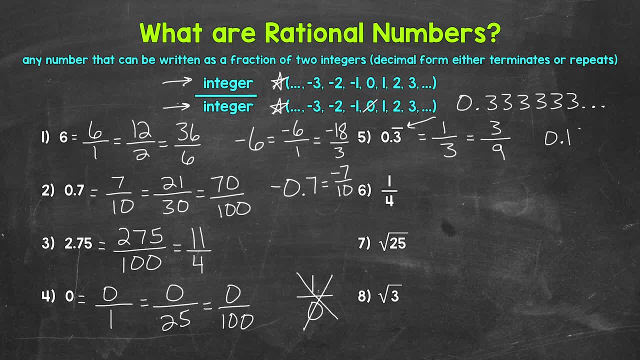 So, for example, something like 0.181818 and this continues on, So 18 repeating. We have a pattern here. We have something that repeats. So this is rational Fractional form. let's come below here, So 0.18 repeating. 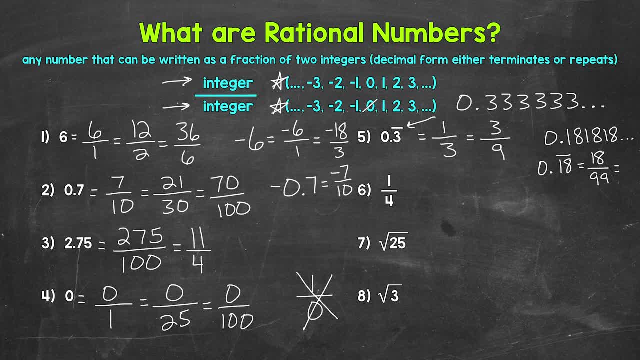 We can do 18 over 99 or even 2 over 11.. Next, for number six, we have one fourth. Well, this is already a fraction. The numerator is 1,, which is an integer, and the denominator is 4,, which is an integer. 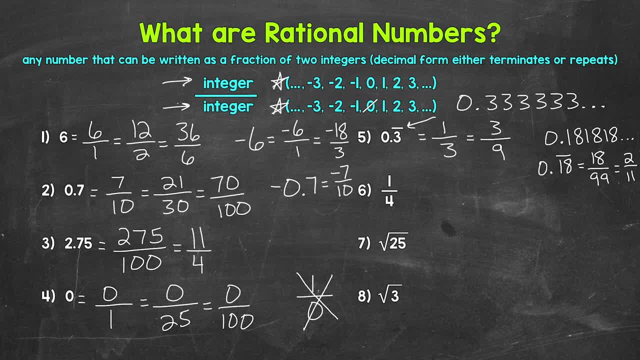 So this is rational. Now let's look at the decimal form as well. One fourth equals twenty-five hundredths, which is a terminating decimal. So we can see that this is a rational number that way as well. Let's move on to number seven, where we have the square root of 25.. 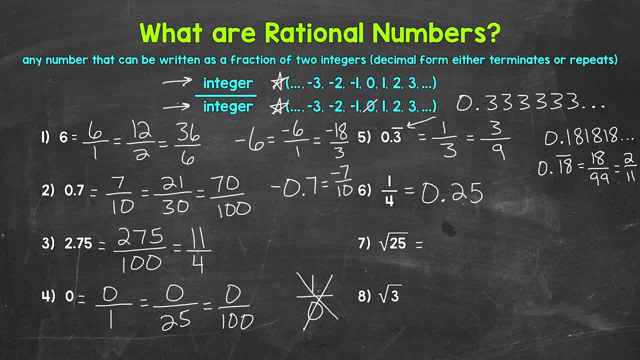 Well, the square root of 25, that equals five. So, with the square root of 25 giving us the value of something like three fifths, we can write this as a fraction of two integers. Now, this is rational, giving us the value of 5, is 5 rational? Yes, 5 is a whole number and we can write it as a. 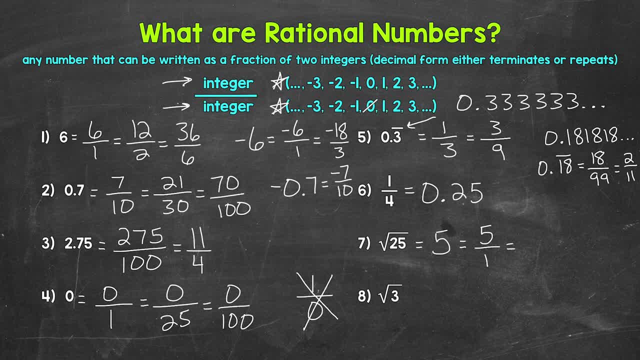 fraction of two integers: 5 over 1,, 50 over 10, so on and so forth. So the square root of 25 is rational. Lastly, let's move on to number 8. And at this point you may be thinking. 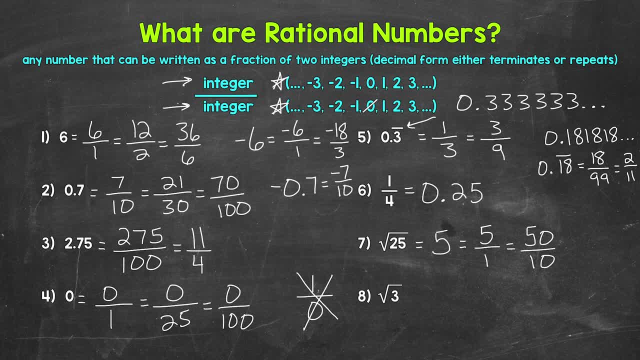 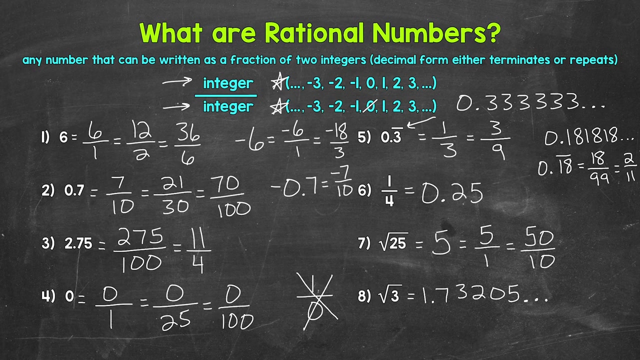 well, what's an example of something that's not rational? Well, the square root of 3 gives us a value that is not rational. If we plug this into a calculator, we get 1.73205, and this continues on forever. Now, this decimal does not repeat, It doesn't have a pattern, And 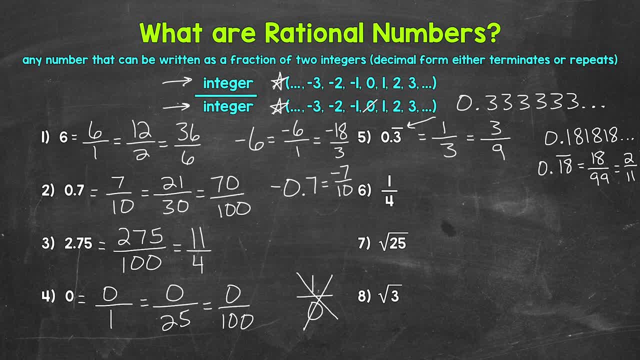 Well, this is already a fraction. The numerator is 1,, which is an integer, and the denominator is 4,, which is an integer. So this is rational. Now let's look at the decimal form as well: 1 fourth equals 25 hundredths, which is a terminating decimal. 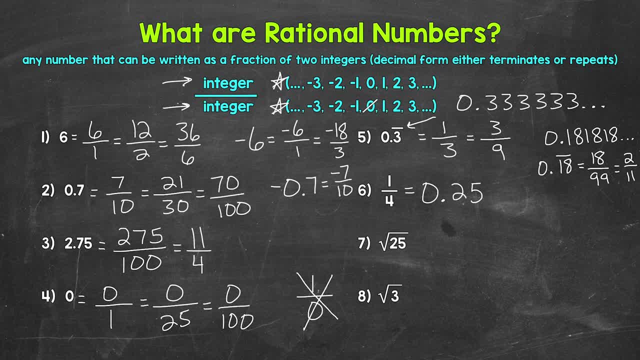 So we can see that this is a rational number that way as well. Let's move on to number 7, where we have the square root of 25.. Well, the square root of 25,, that equals 5.. So, with the square root of 25 giving us the value of 5, is 5 rational. 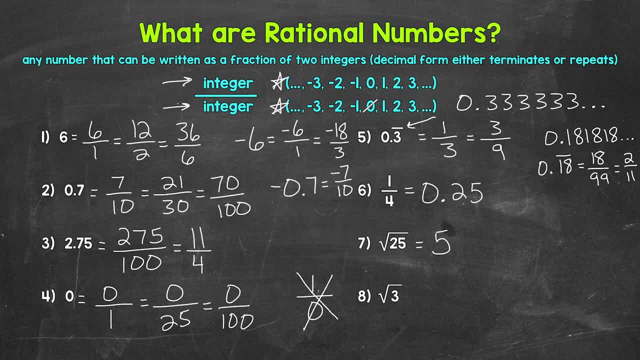 Yes, 5 is a whole number and we can write it as a fraction of two integers: 5 over 1,, 50 over 10, so on and so forth. So the square root of 25.. 5 is rational. 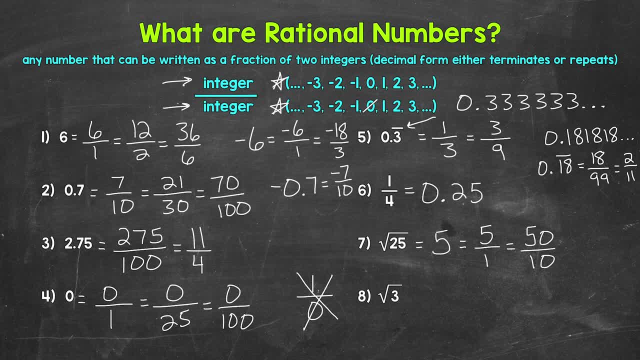 Lastly, let's move on to number 8.. And at this point you may be thinking: well, what's an example of something that's not rational? Well, the square root of 3 gives us a value that is not rational. 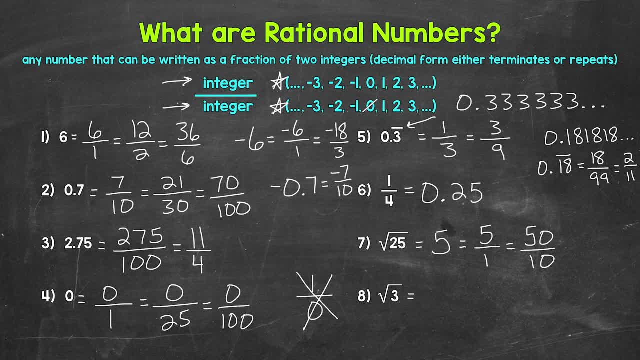 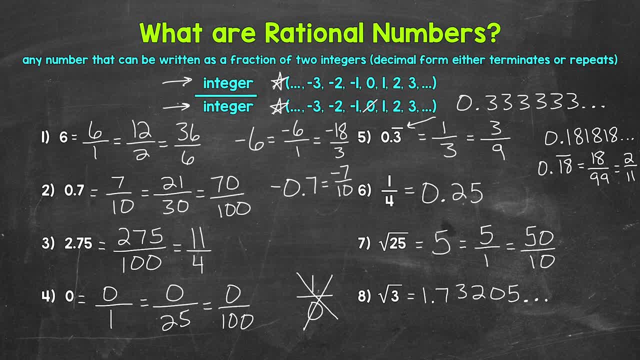 We're going to get a perfect answer, But this decimal does not repeat, It doesn't have a pattern And again, it continues on forever. So the decimal form doesn't terminate or repeat. So there is no way for us to write this as a fraction of two integers. 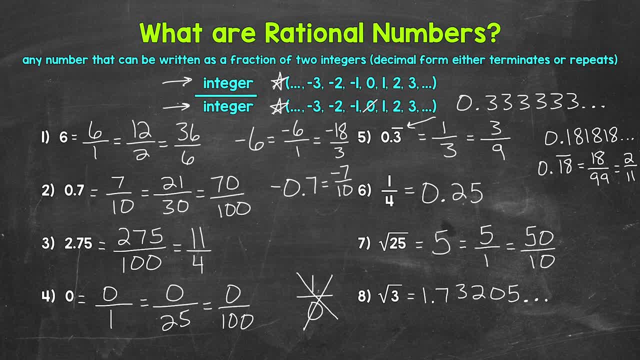 So this is not rational. Again, there's no way for us to write this as a fraction of two integers. But you may be thinking: can't we just write this as the square root of 3 over 1? That's a fraction. 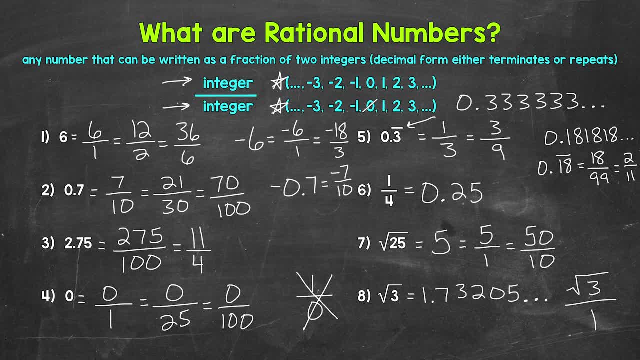 Yes, it is a fraction, But remember, a rational number is any number that can be written as a fraction of two integers And this numerator is not an integer. Again, the numerator and denominator have to be an integer for it to be rational.